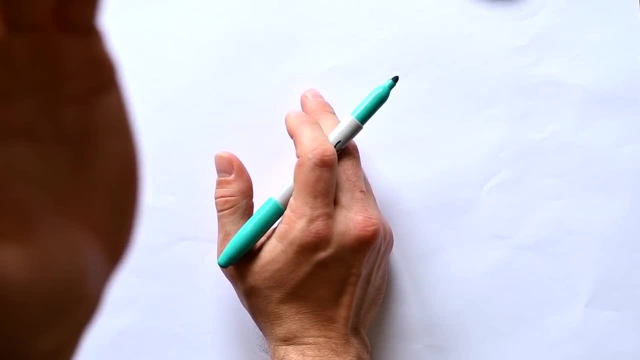 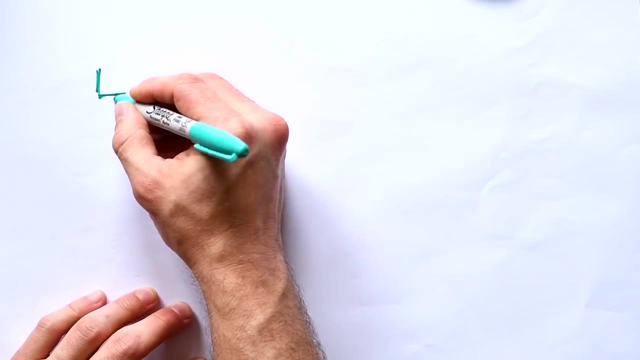 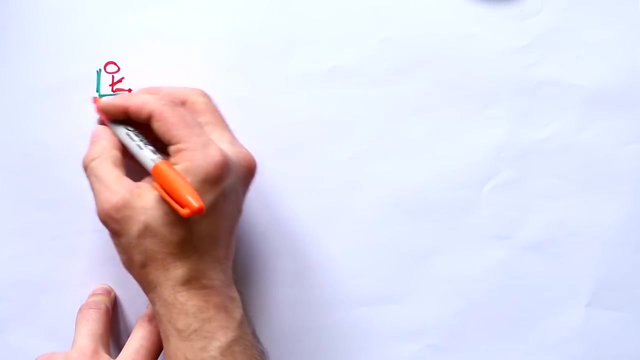 Okay, this is rotational dynamics, or in other words, the physics of spinny things. Now, I'll always remember when I was a kid, my dad used to put me on a spinny swivel chair and I used to sit there like that with my legs down, and he used to spin me like that. 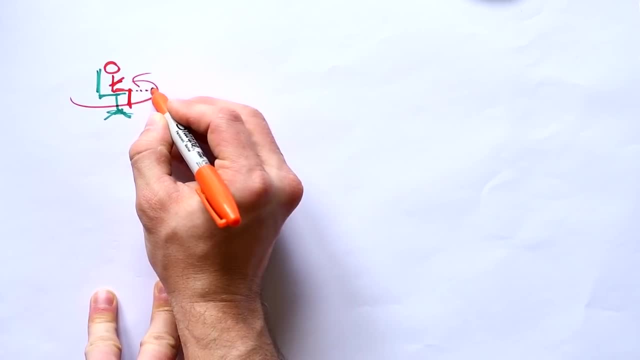 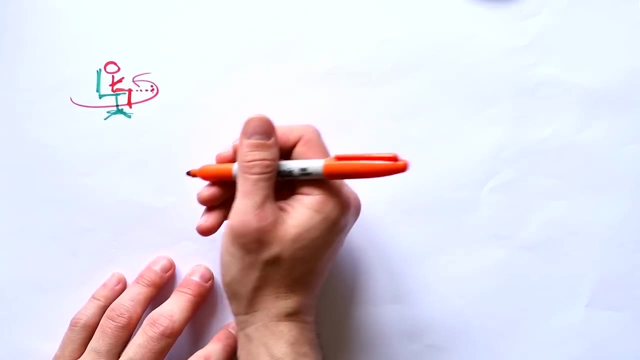 What he said was: stick your legs out, And what I realized was, when I stuck my legs out, I went slower. When I tucked my legs back in, I spun faster, And that is all to do with what we're talking about today. So the first thing that you need to know is the concept of moment. 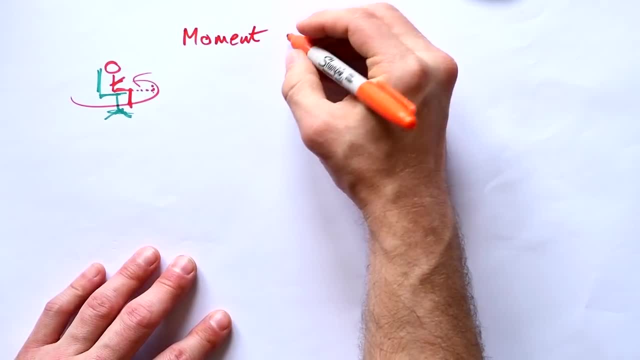 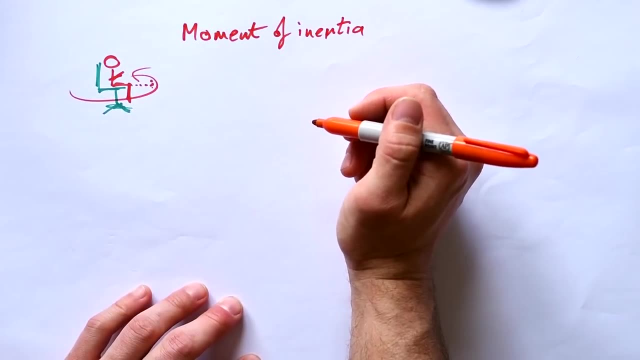 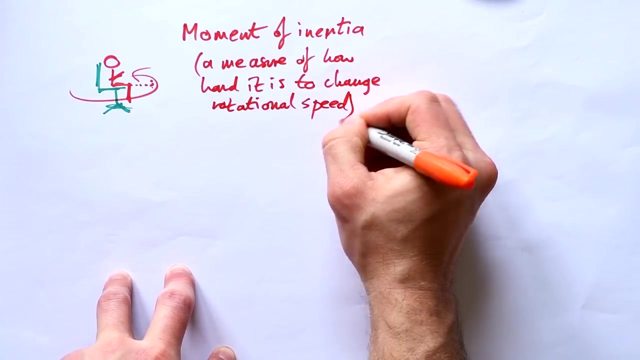 of inertia. Now, everything in rotational dynamics has a sort of counterpart in linear dynamics. So you know just your suvat Now moment of inertia. it's a measure of how hard it is to change rotational speed. You might call that angular speed as well. We'll get on to calling it that. 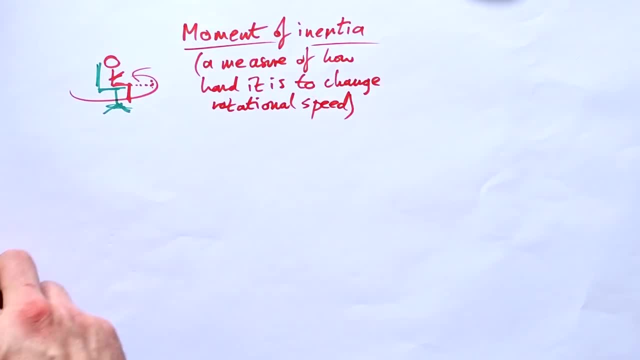 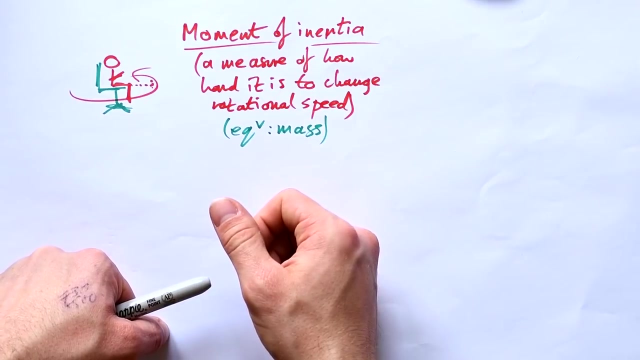 later. But this idea of moment of inertia, we can think of that as mass. So the equivalent- I'm just going to write equivalent, as that is mass. So if you have something that has a heavy mass, then it's harder to change the speed of it, In other words it's more resistant to changes in. 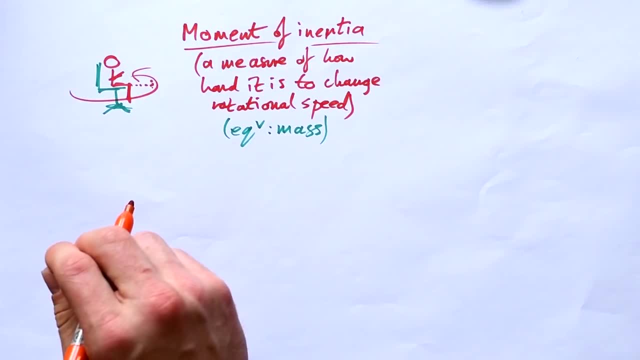 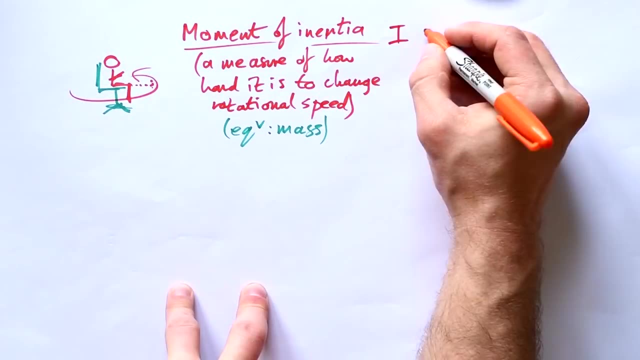 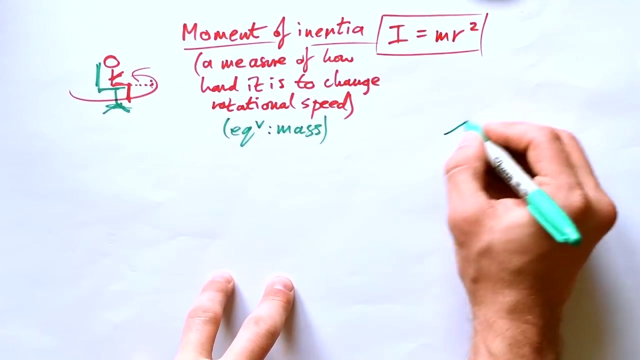 speed than something that's lighter, And it's the same thing with moment of inertia. This is, given the symbol capital, I, not to be confused with impulse. And this is equal to m r squared. This is true for maybe a conker on a piece of string. 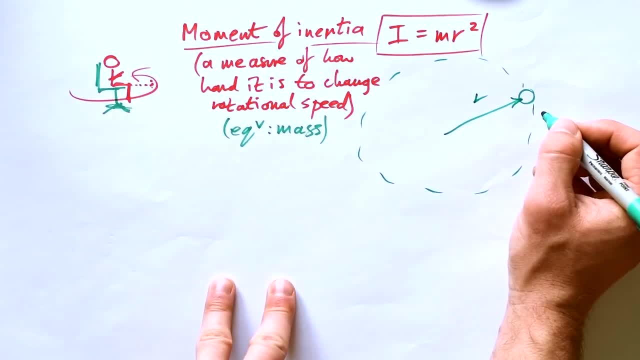 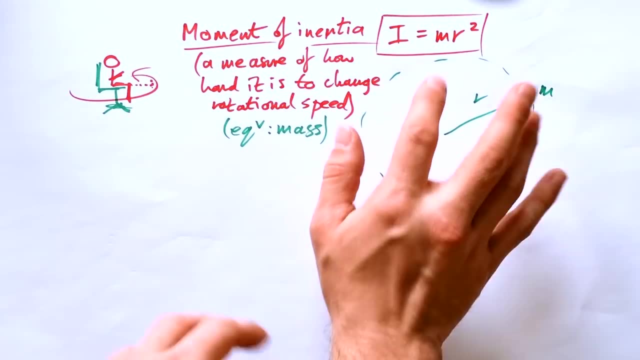 Let's go around in a circle. The length of the string is r and we have a mass. This is true for point masses. So there's no mass in between. Now, that's something that you have to know, as it were, But this changes for when we have, say, a ball. 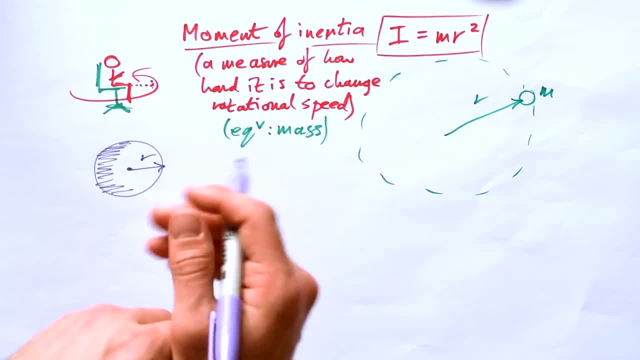 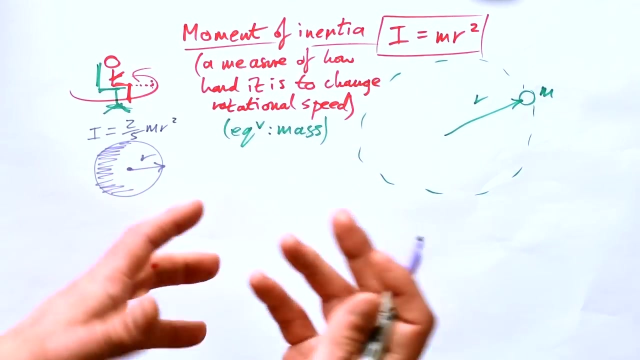 So if we have a ball that's spinning, obviously not all of its mass is on the outside And also the mass is evenly distributed in all directions. In this case, a sphere's moment of inertia is equal to two-fifths m r squared. You don't need to know where you get that from, That's. 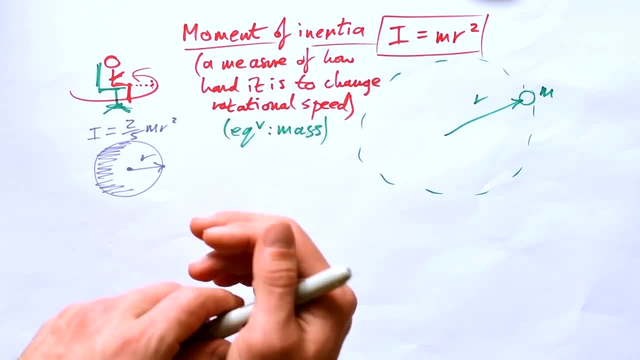 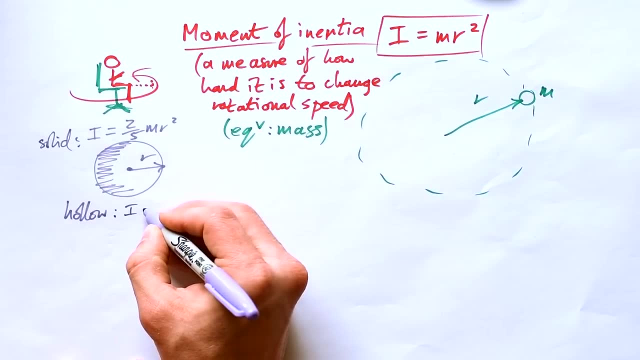 something that you might do in maths, But we don't need to know how to do that in A-level physics. If it's a hollow ball, then it's slightly different. So that's for solid. If it's a hollow ball, then the moment of inertia is equal to two-fifths m? r squared. So that's for solid. 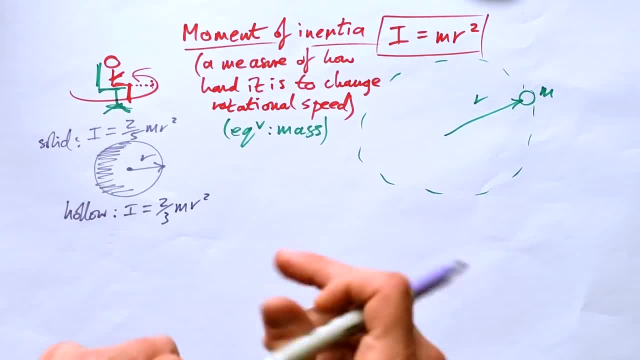 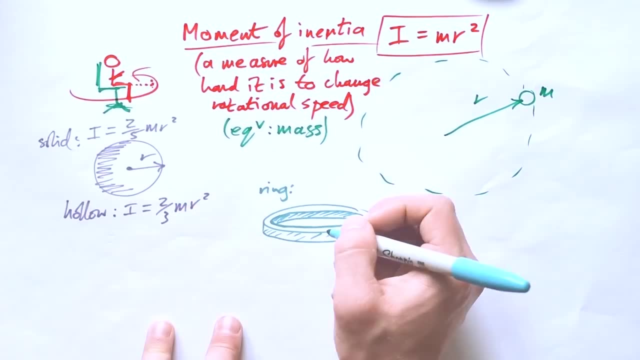 The moment of inertia is equal to two-thirds m r squared Of course, the m being the total mass of the sphere, whether it's solid or whether it's hollow For a ring. it's fairly easy, because the moment of inertia is again going to be m. 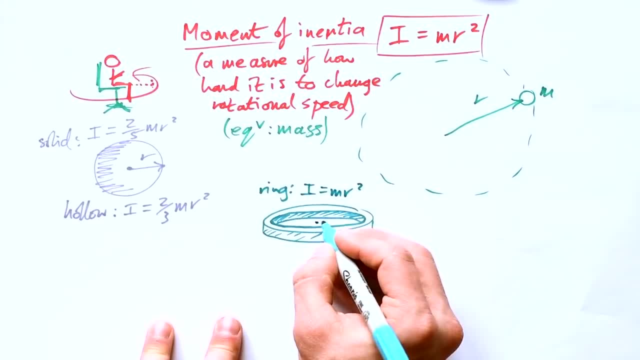 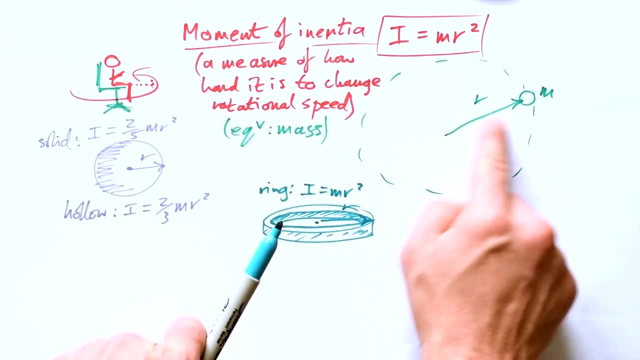 r squared, And that's because all of the mass is at the radius as well. There's no mass in the middle at all, And so we'll get onto how that works with that in a minute. But if it's a solid disc, 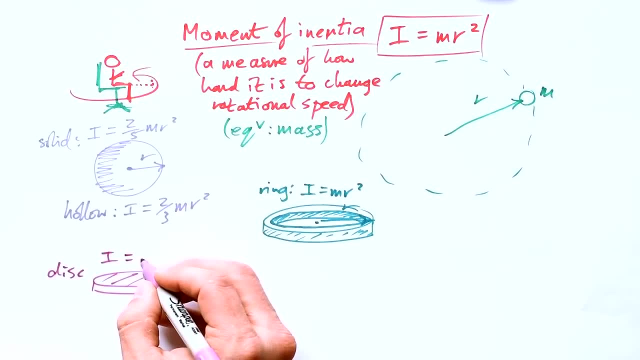 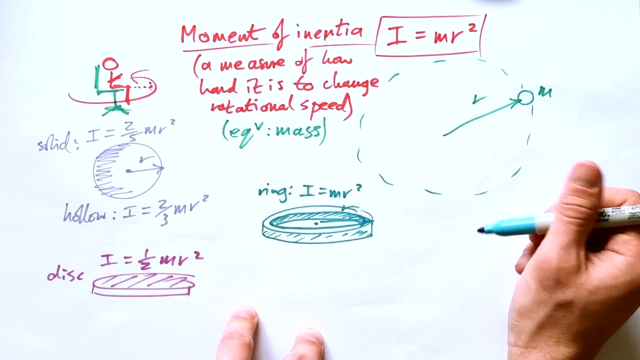 then the moment of inertia is a half m r squared. Like I said, you don't need to know these off by heart. You'll always be given those in the exam. Now, the reason that the moment of inertia is the same for a ring as it is for just a mass on the end of a piece of string is because total moment. 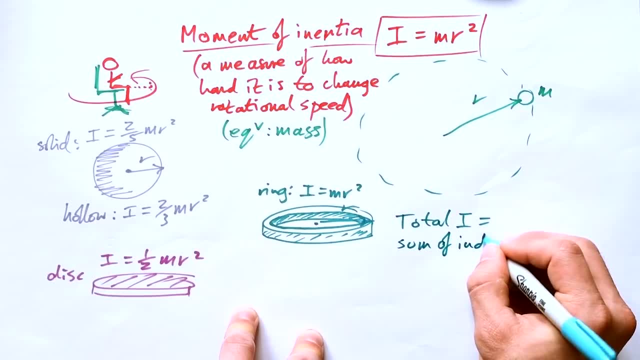 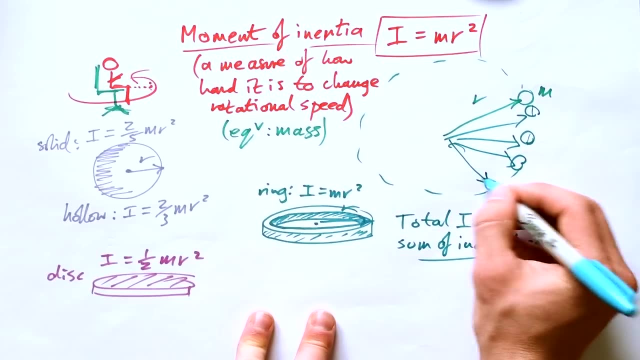 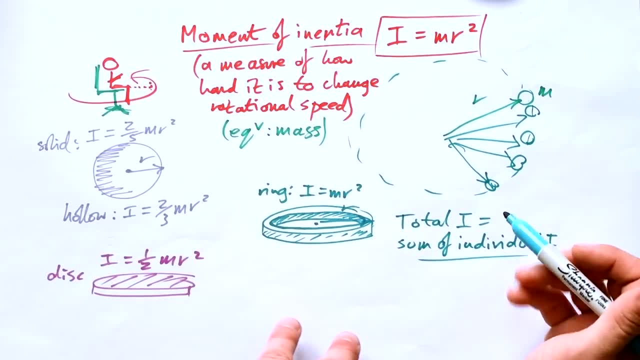 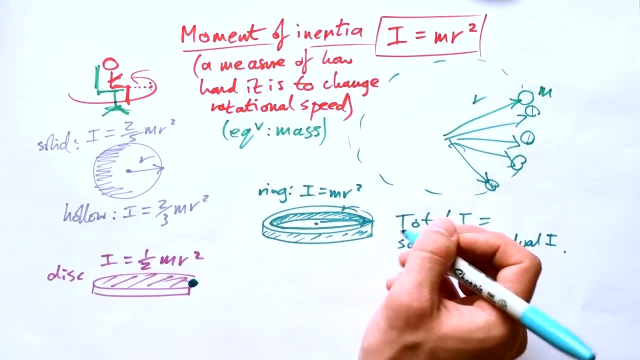 have in essence then is just a ring. But that's super important: that if you add something else onto something- maybe you put a mass on the end here of a disc- then the total moment of inertia of this disc is going to be this plus m? r? squared for this particle on the end. 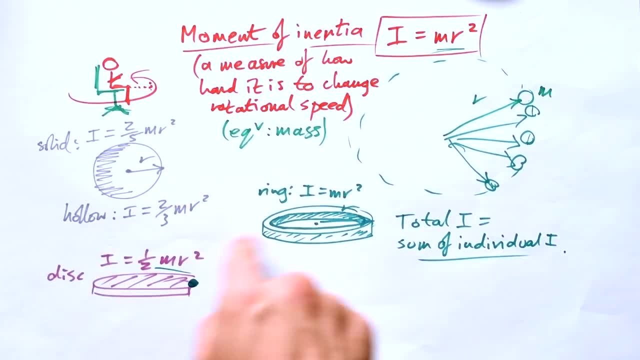 You can add them up. More often than not, it's going to be one of these plus a particle, So you're just adding on m r squared to get the total moment of inertia. Now, with linear dynamics, we're talking suvat, aren't we? So s? do you know what I'm going to leave out? u because we're not really. 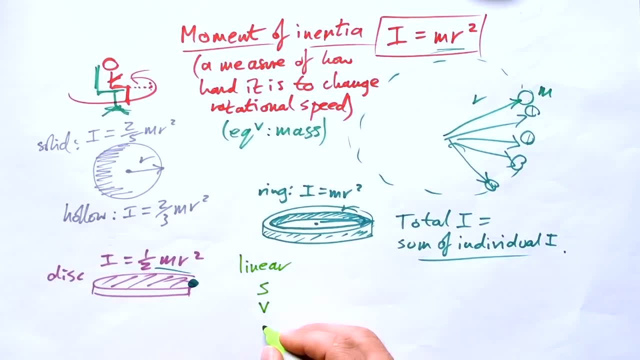 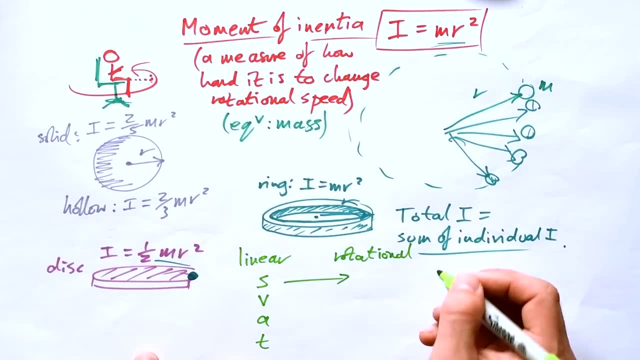 concerned with that. I'm going to call that v, because u and v are the same. We have a and we have t. t is going to stay the same. Time doesn't change whether it's linear or rotational, But rotational. there's no such thing as displacement, as it were. What's the only thing we're concerned? 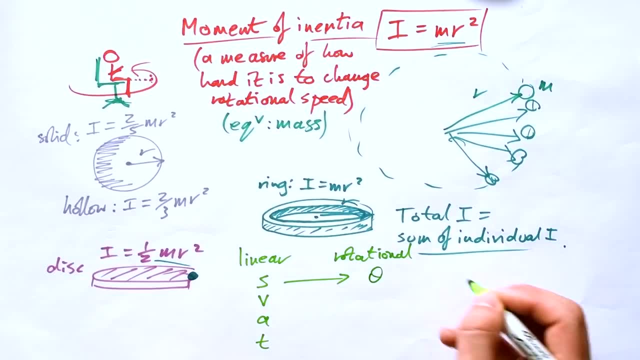 with when it comes to going around in circles, We're talking about the angle that we go through. If you think of displacement for linear, then the equivalent for rotational dynamics is the angle. Of course we have to be working in radians. Linear speed is meters per second. Rotational. 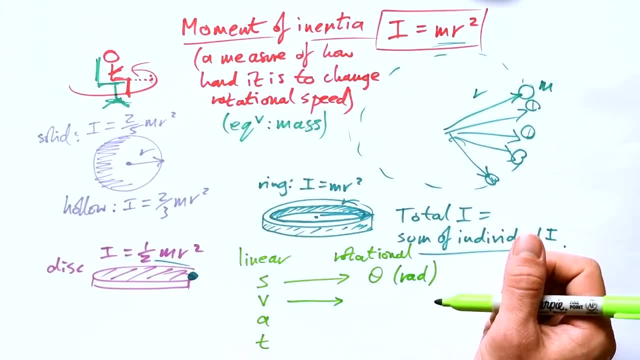 well, we're covering a certain angle in so many seconds, So we're going to be degrees per second. No, We use angular speed omega for rotational dynamics And anything going around in a circle, don't we? Especially when it comes to SHM and circular. 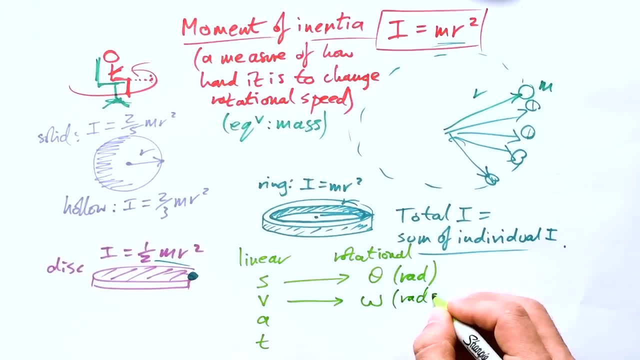 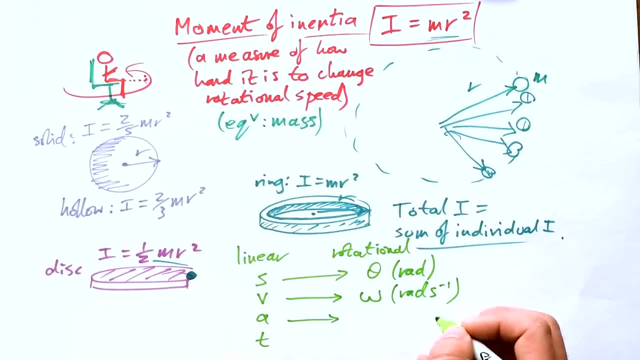 motion as well, And so this is going to be radians per second Acceleration. this is similar, But of course it's not going to be meters per second squared, It's going to be radians per second squared. So we do give it a different symbol, We give it an alpha instead. Similar, but not the same. 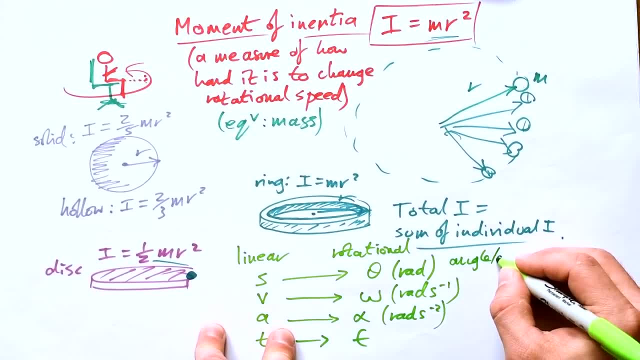 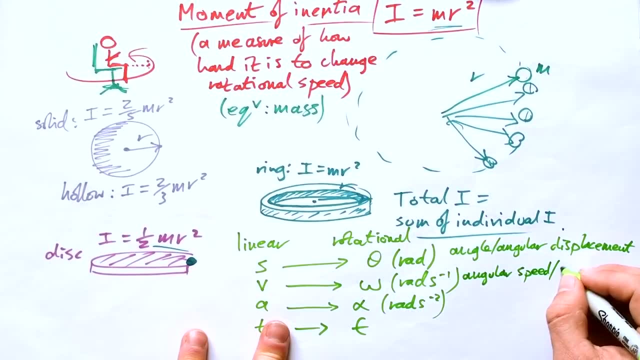 And then we have time as well. That just stays the same. We can also call that angular displacement. So how far around a circle? Well, have you gone? Angular speed- sometimes we call that angular frequency And, of course, angular acceleration. And, like we said, mass. well, the equivalent is moment of inertia, And 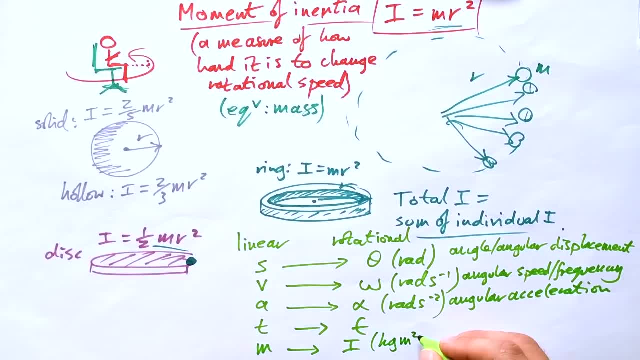 the unit of this is, of course, going to be kilogram meters squared, And the reason that we're talking about the similarities between linear and rotational dynamics is because, basically, all of the laws that apply for linear dynamics also apply to rotational as well. 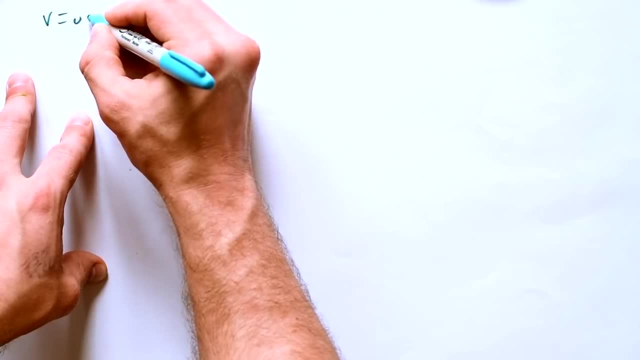 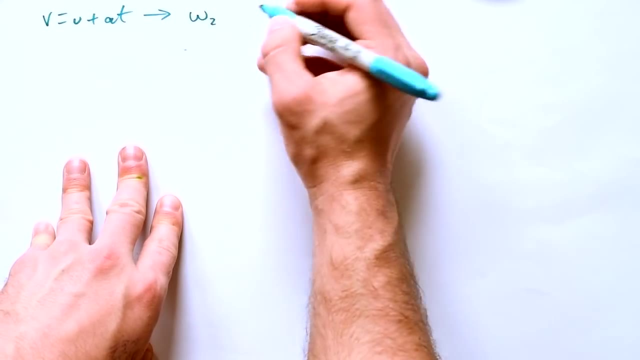 Well, let's think about Newton's equations. This is a motion. v equals u plus at. What would the equivalent be for rotational dynamics? Well, just a second speed is equal to the first angular speed, that is, plus angular acceleration times. 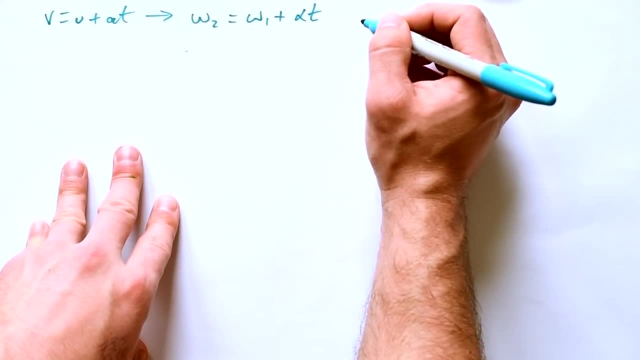 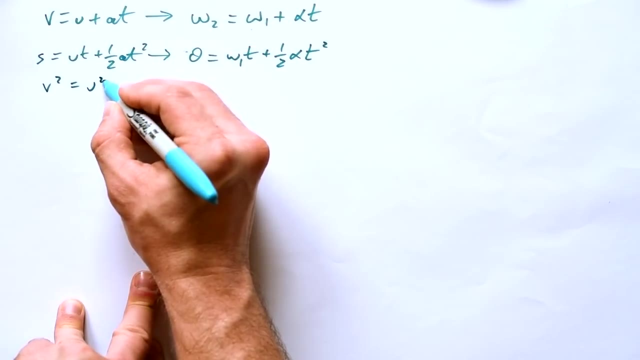 time. It's exactly the same, just we're thinking circles, not lines s- equals u2 plus half at squared. You can figure this out yourself. I reckon v squared equals u squared plus 2as. And the last one as well. Pretty nifty right. 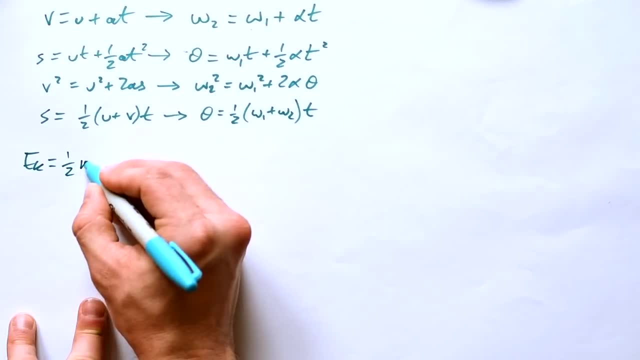 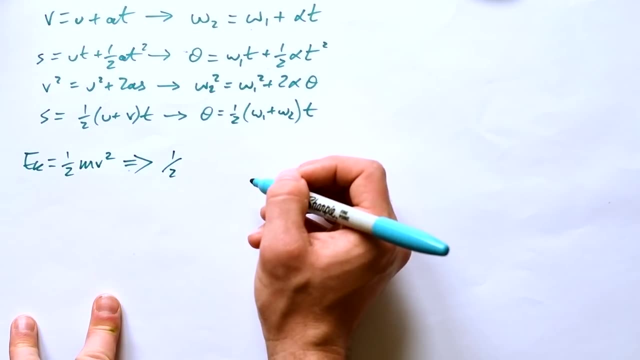 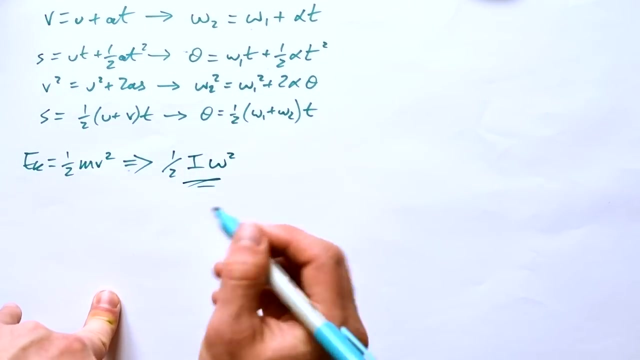 Even things like kinetic energy. We know that ek is equal to half mv squared. The equivalent for rotational dynamics is half, And we said that the equivalent to mass is the moment of inertia. And then we just times by our angular speed squared, So that gives you the 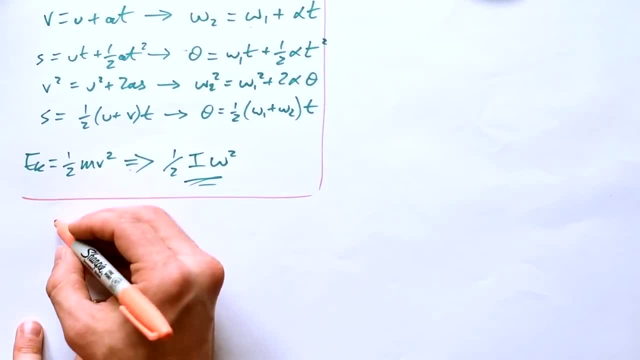 kinetic energy of a spinny thing, And let's have a think about torque, In other words moments. you can call them that as well. Torque is a nicer word to go with And we're going to call that T for torque. 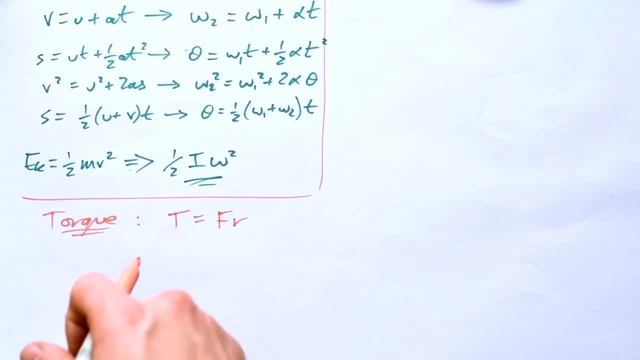 And torque is the moment of inertia, times the distance that that force is from the pivot, And the unit of that is going to be Newton meters. Of course, these need to be perpendicular, don't they? But what you might not know is that it is also equal to the moment of inertia of the thing that's. 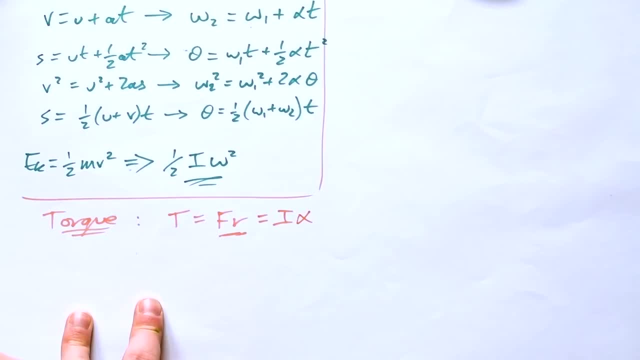 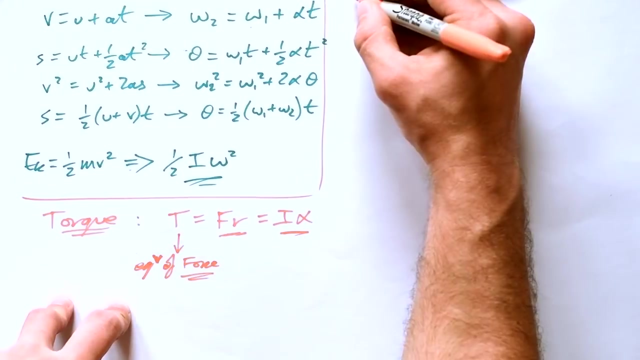 being turned times the angular acceleration. So in other words, torque is equivalent of force- because it's our moment of inertia- times angular acceleration that it is the equivalent to force. when it comes to rotation, We have work done as well. You know that work done for something going in a line is just E. 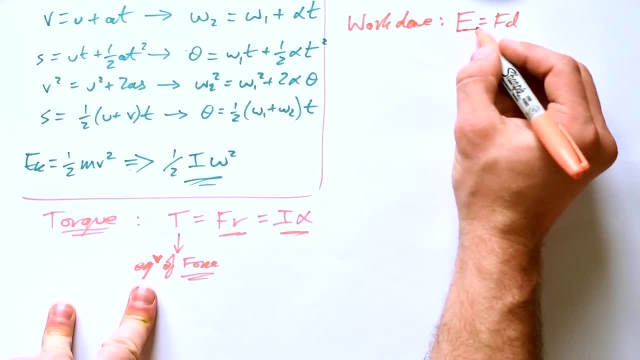 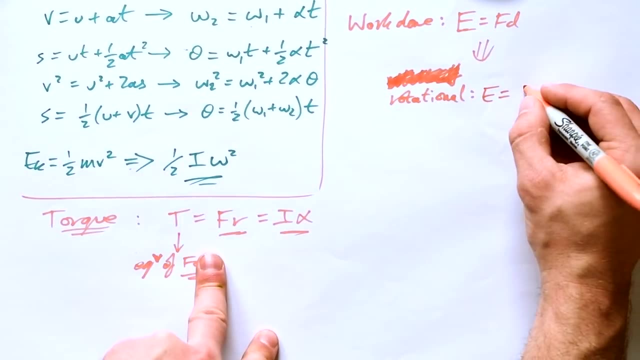 equals FD. I don't like using W, it's an energy. So E equals FD. But what would it be for rotational? Well, we said that the equivalent to force is our torque. So let's take our torque and we need to size it by a distance, but we don't deal. 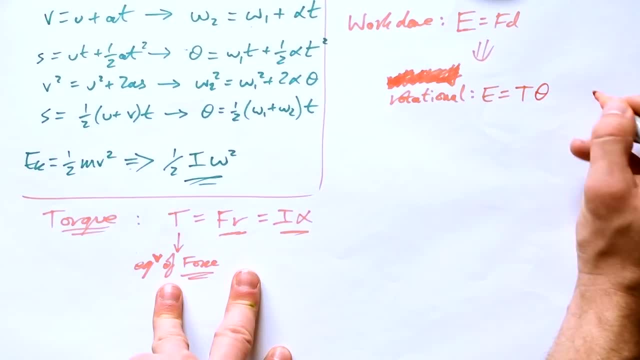 with displacements or distances. we deal with angular displacement, And so that's how we find the work done by something that's turning Torque times the angle that it's turned through. We can go with power as well. We know that power is P. 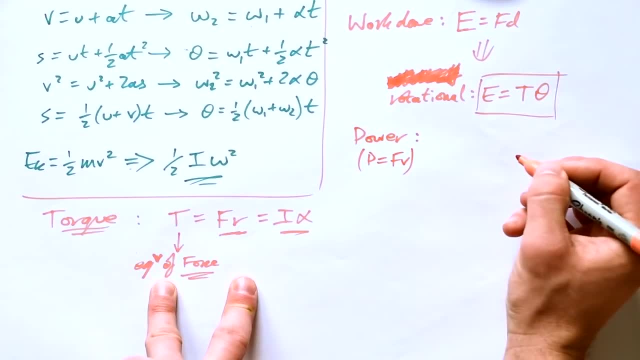 equals FV for something that's only going in linear motion, And so therefore, we can say that let's take our torque and times by speed, but that's going to be angular speed. So that's the power Which makes sense, because we just get from here to 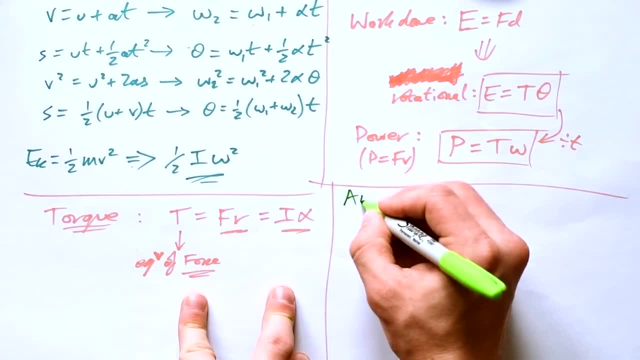 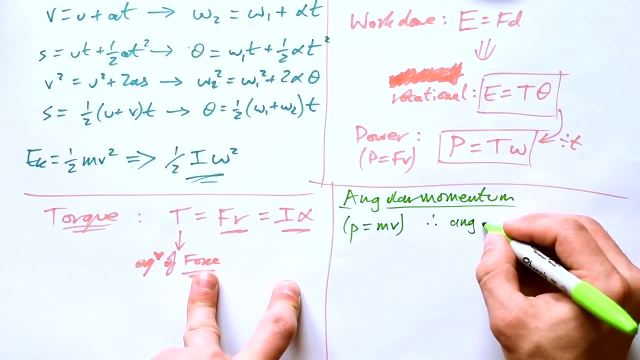 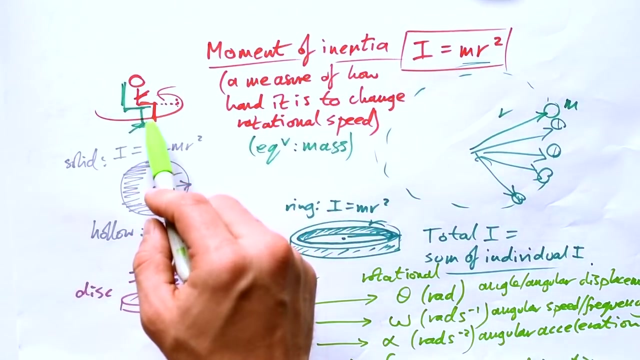 here by division. And finally we have angular momentum. We know that linear momentum is just equal to MV, So therefore angular momentum is equal to our equivalent. that's our moment of inertia times. angular speed And, just like normal momentum, this is always conserved. So let's think back to me on the spinny chair here. What is? 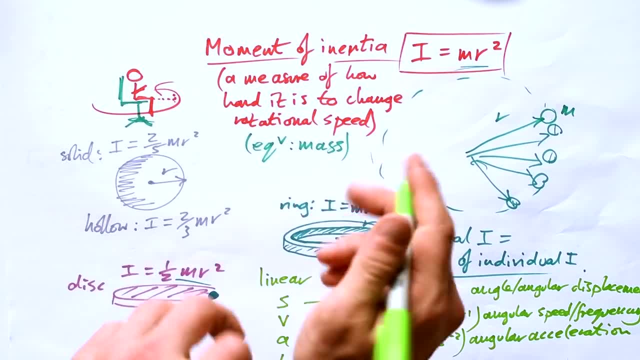 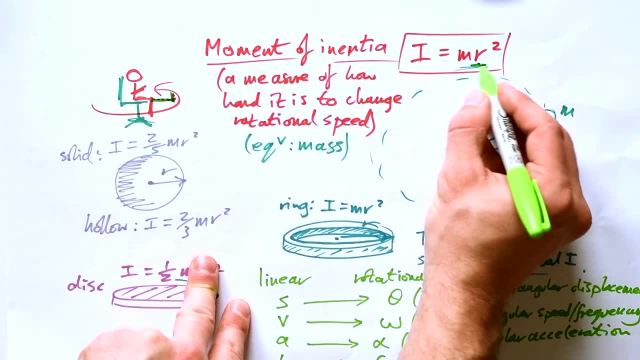 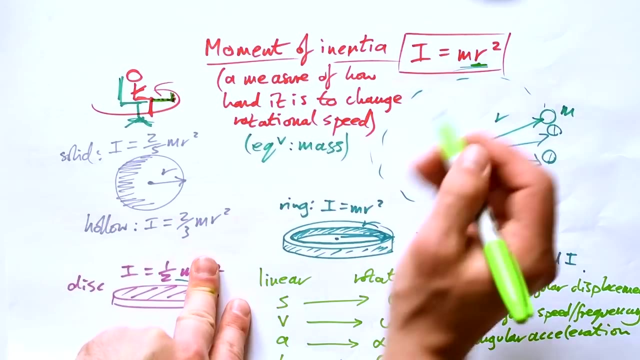 happening when I pull my legs in from when they were sticking out like that. So if they were sticking out and then I bring them in, I'm actually decreasing the distance that the mass is from the pivot. So I'm decreasing ourário from decreasing 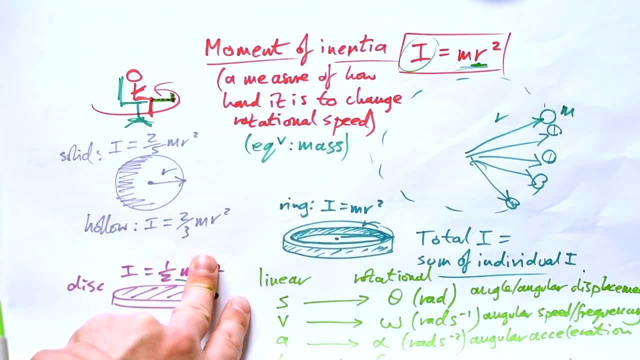 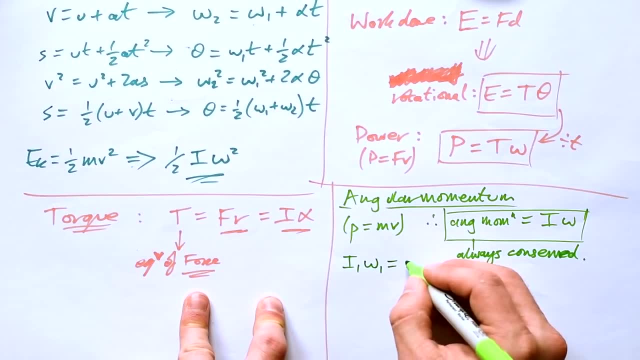 Rr, then the moment of inertia decreases as well. If we know that angular momentum is always conserved, then we can say that I1 omega 1 is equal to I2 omega 2.. So if I'm decreasing, or we can say that, 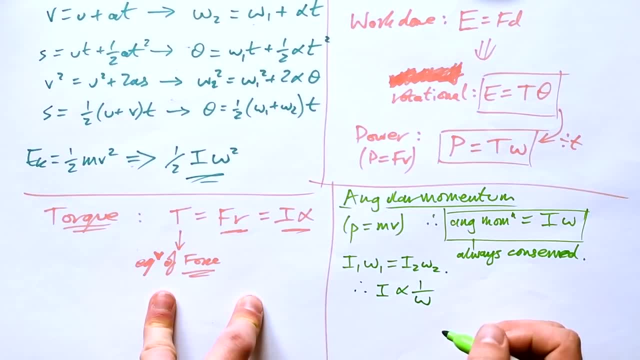 is inversely proportional to angular speed, and we can put it the other way around as well. So that means that if my moment of inertia is going down because I'm bringing my legs in in order for angular momentum to be conserved, that means that my angular speed goes up. So that's why you spin faster. And, of course, 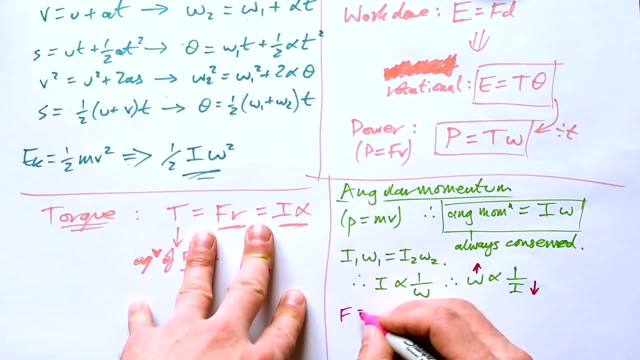 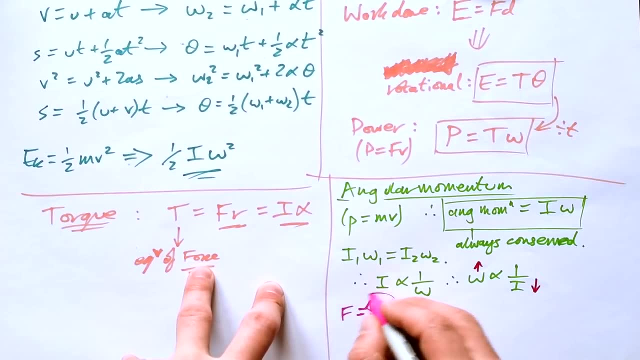 we know that force is equal to the rate of change in momentum, don't we? So that's equal to delta mv by T for something undergoing linear, And we know that this is our impulse, and so that means that for rotational we have angular impulse. 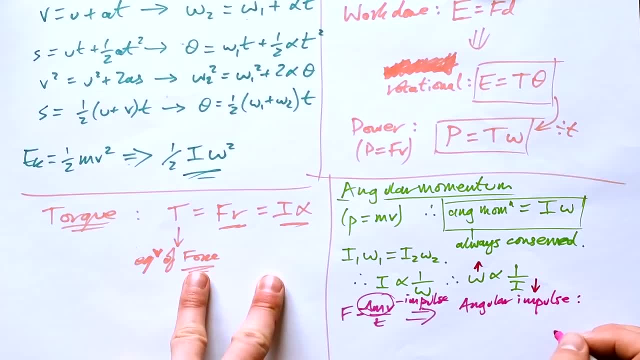 I'm not going to put capital I because you don't want to get confused. Angular impulse is going to be equal to. similarly, delta i, omega m goes to moment of inertia. speed goes to angular speed. But we know that for force the equivalent for that is torque. So that means that our torque is equal to. 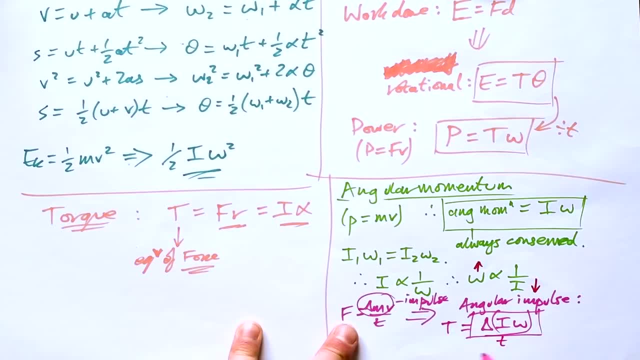 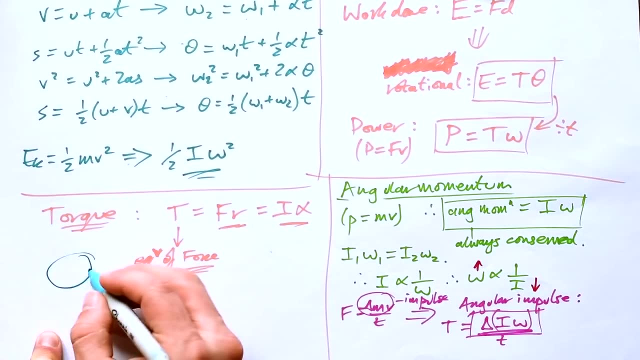 the angular impulse divided by the time. Quite often the hardest questions that you'll get is when you have, say, a wheel that is maybe lifting a mass, or rather the mass is falling down and it's spinning the wheel. Um, what you've got to? 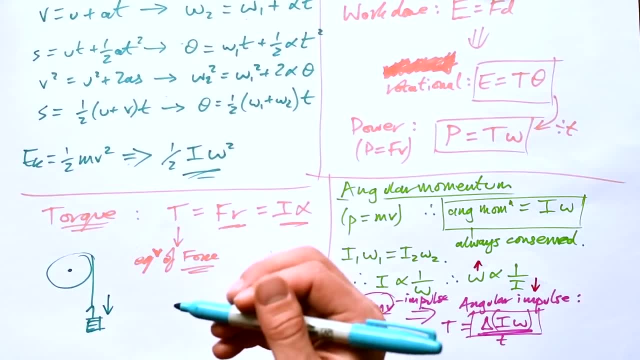 remember. what you've got to think about is right: what energy is going to be being created? So certainly, whether the variable is the do I have here. If a mass is falling, then that means that the only energy to begin with is mgh. What is that being transferred to? Well, that's being 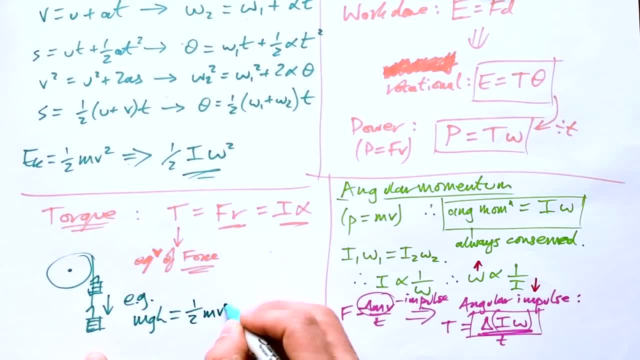 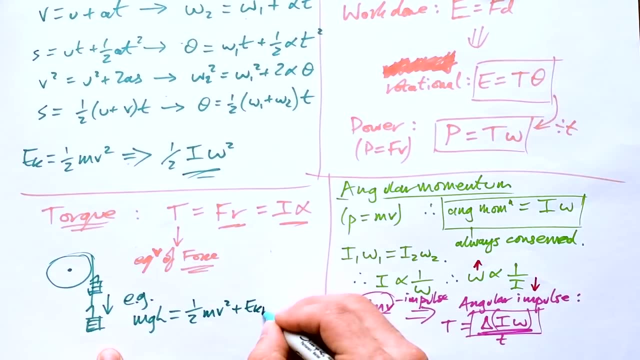 transferred to the kinetic energy of the mass there. so that's just half mv squared. That's also being transferred to the ek of the disk. I'm just going to put ek rotational and we know that that is equal to half i omega squared. and if 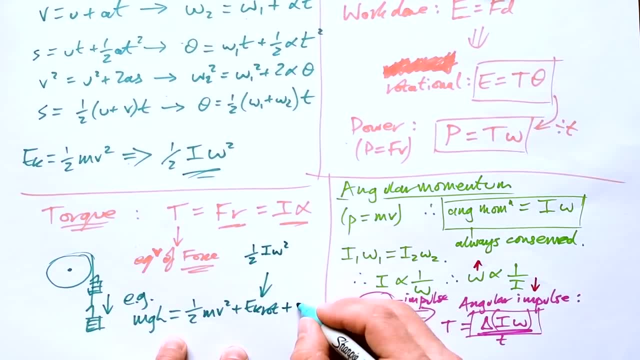 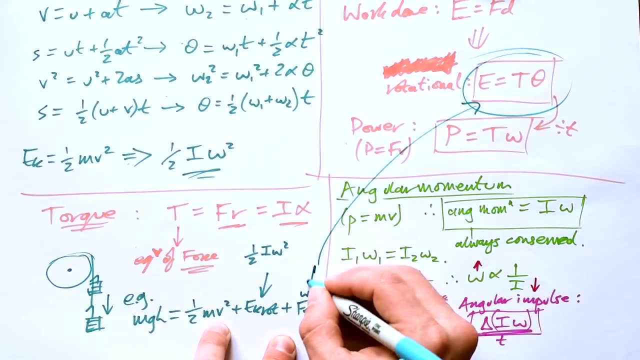 there's no friction involved, then that's going to be it, but then if there is friction involved as well, if there's work done against friction, then we know that that's this one up here, and so we can say that that is the torque times theta. One more thing that you might need to know is about flywheels. Now, flywheels. 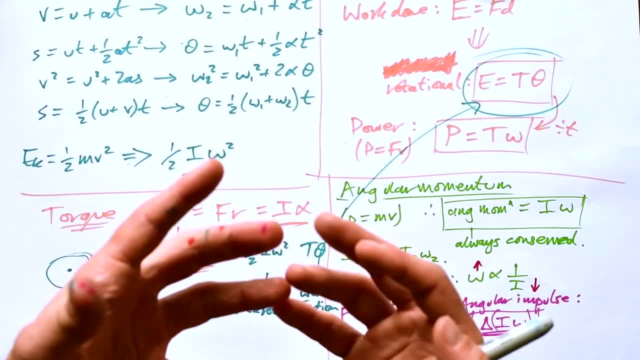 have been around for a long time. they're using lots of things, but they're things that we're not starting to see. So, for instance, let's imagine that we have a small workshop that's not focusing on a small work system in this class and we 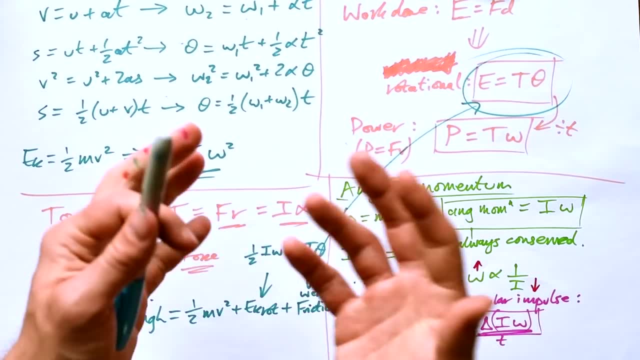 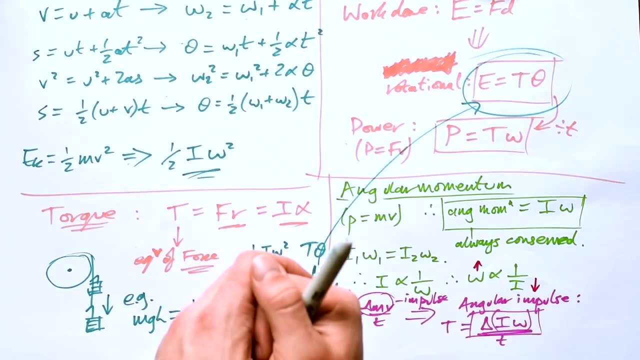 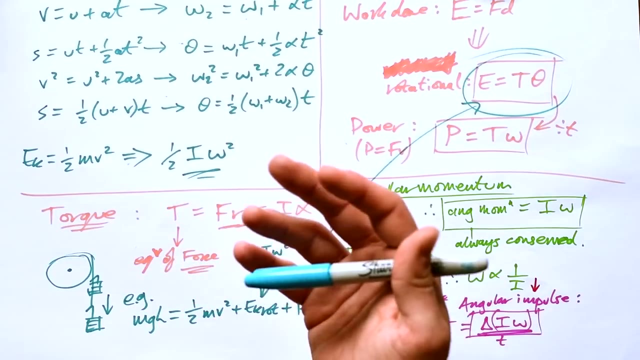 thinking about using flywheels as an alternative to batteries in cars. what you do is that you get a really heavy disc of metal, spin it up really, really fast and then, as you start driving, then that makes contact with the shaft in your car and then that drives the wheels, and so you're taking energy out of that. 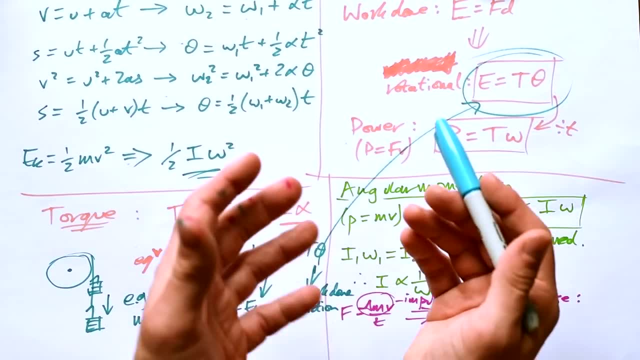 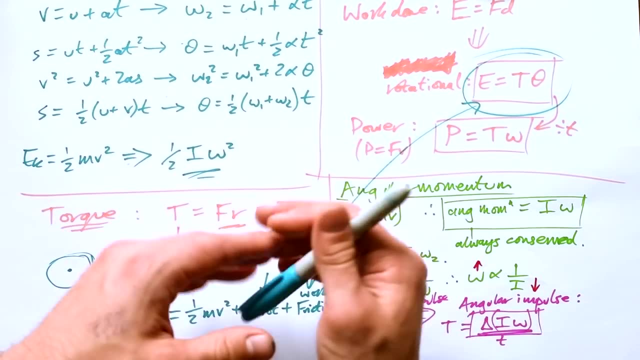 spinning disc little by little, and a good thing about them is that they don't take a long time to charge, because of course you just spin it up, whereas with a battery have to wait for maybe half an hour to charge the battery up, in this case you just start spinning it and that takes, well, just a few seconds to be. 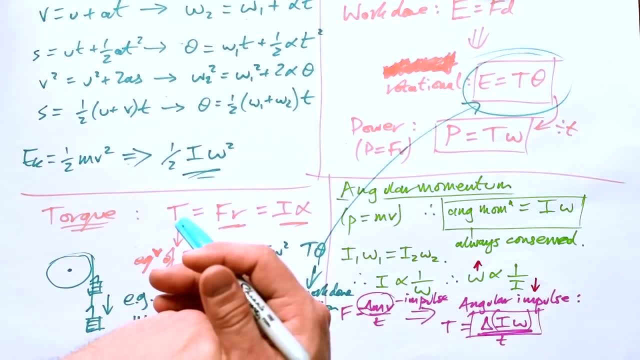 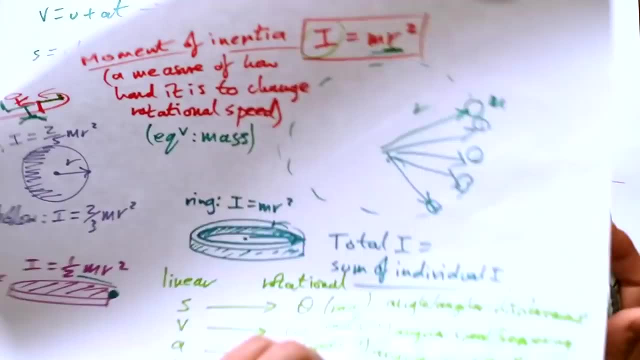 honest, maybe a minute. if it's heavier, then you can store more kinetic energy in it. of course, that does make the car itself heavier as well. so it's a bit of a pro and a con at the same time, and also if you use a ring instead of a disc. 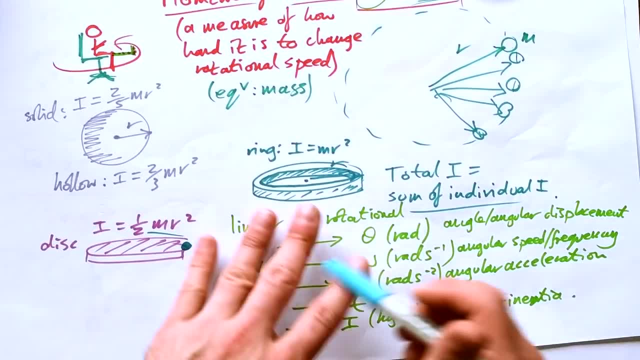 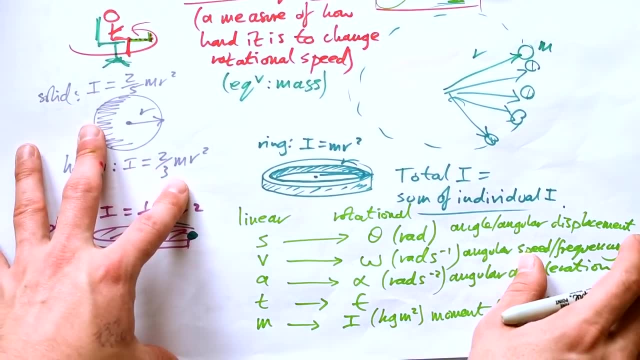 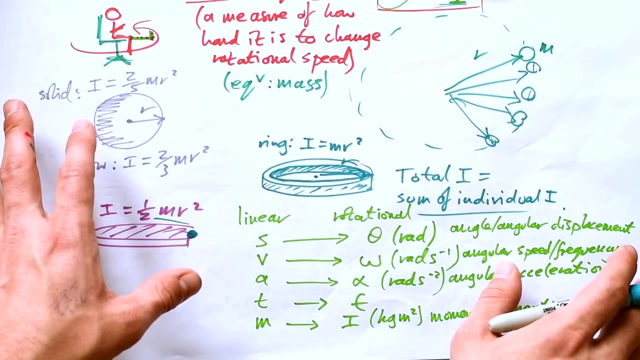 then that means that you have a greater moment of inertia, so that means that again you can store more kinetic energy in it. at the same time, For a flywheel you need incredibly good bearings, because you want as little friction as possible. that's, of course, where lots of energy is going to be lost. 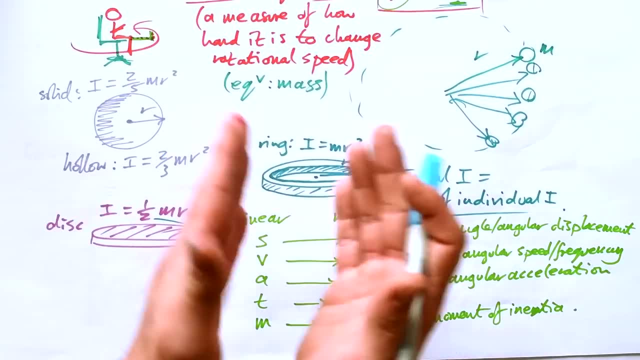 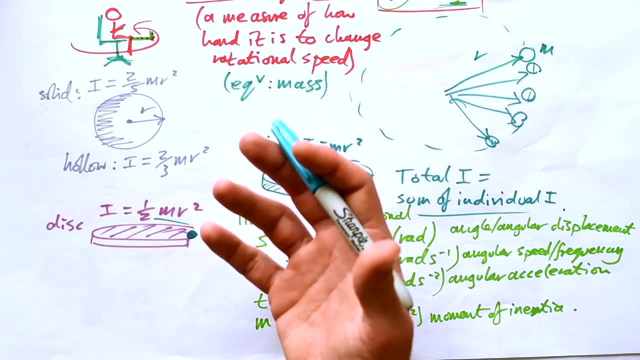 you can't stay charged forever, as it were. it's going to lose energy over time, even when you're not using it. and because there's so much energy in this flywheel, if something breaks and it spins apart now, that's a lot of damage. another application of angular momentum and rotational dynamics is with governors.